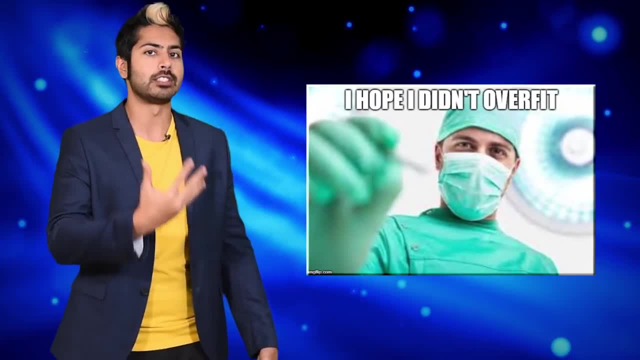 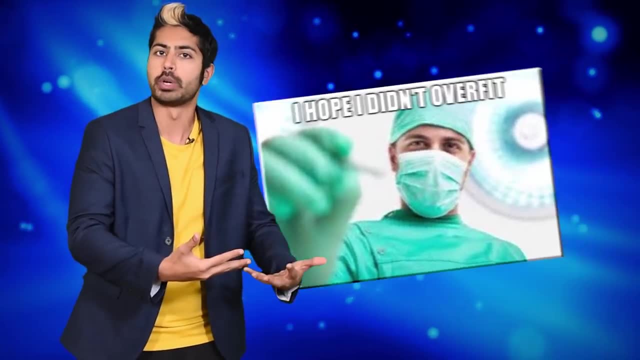 The lead surgeon asked us to use unsupervised learning techniques on this neural data to find out what part of their brain is causing the seizures, so they can perform surgery on it. Will we save the patient's life? We'll find out at the end of this video and subscribe if you want. 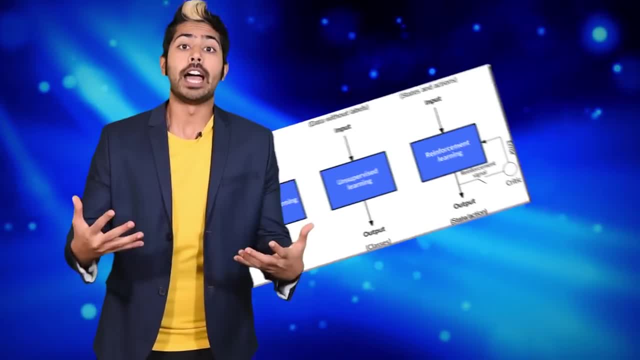 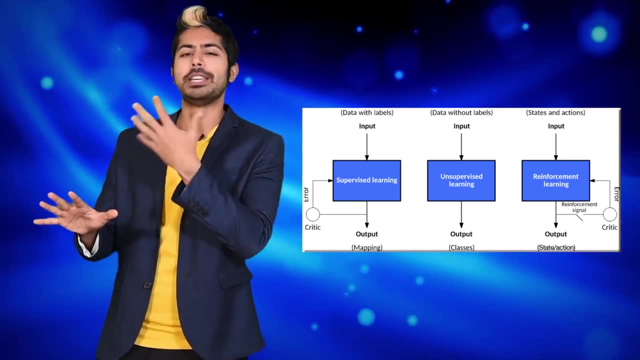 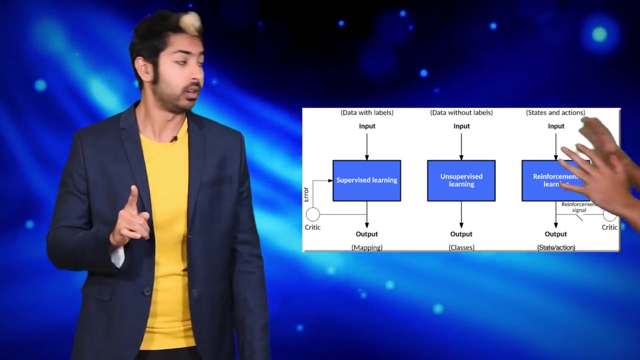 to keep learning about AI technology for free. We can divide machine learning into two types: supervised and unsupervised. There's also reinforcement learning, but that only applies in a real time environment. It's not a static data spreadsheet. There's also quantum machine learning. Can you please keep it simple? 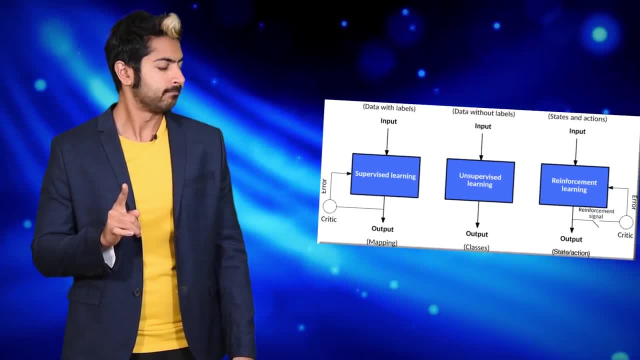 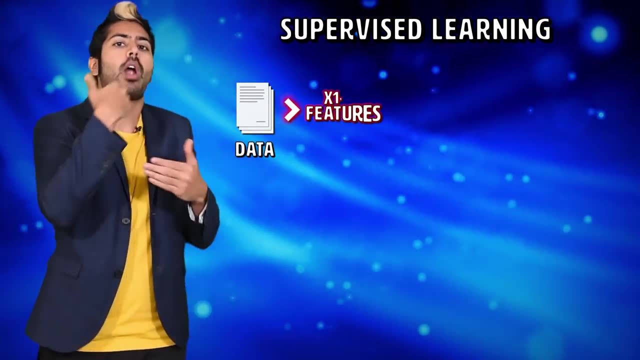 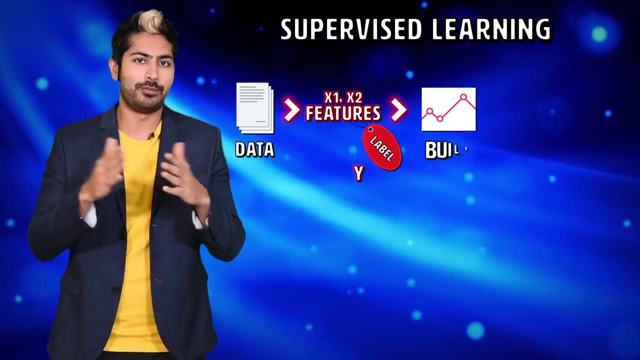 for once, Supervised learning is synonymous with pattern matching. It's done using the ground truth, meaning we have prior knowledge of what the output values for our input data should be. You know that hot dog, not hot dog classifier- trope from the popular show Silicon Valley. 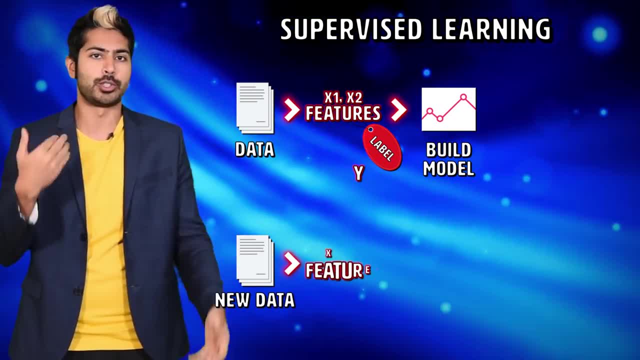 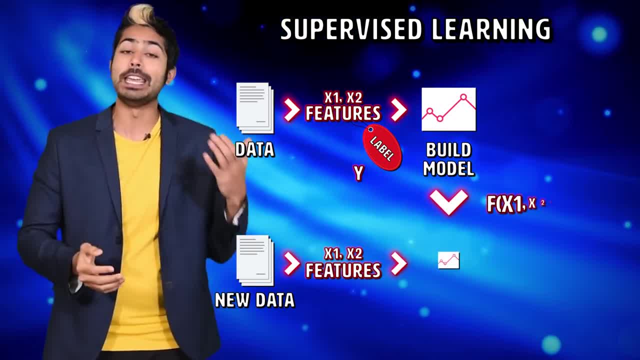 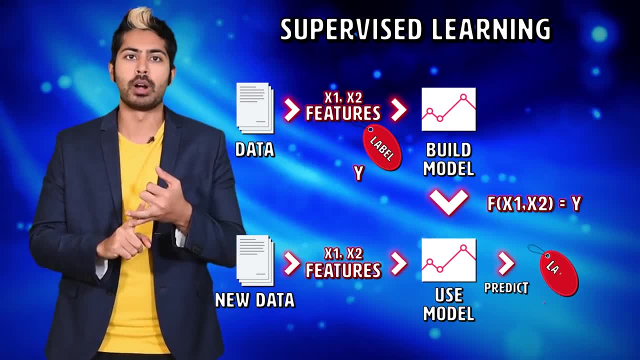 The goal is to approximate the relationship between input and output data. Most machine learning across every industry is done this way. It's easy, it's straightforward and it tends to perform very well, if given enough examples. But clean, perfectly labeled data sets aren't always. 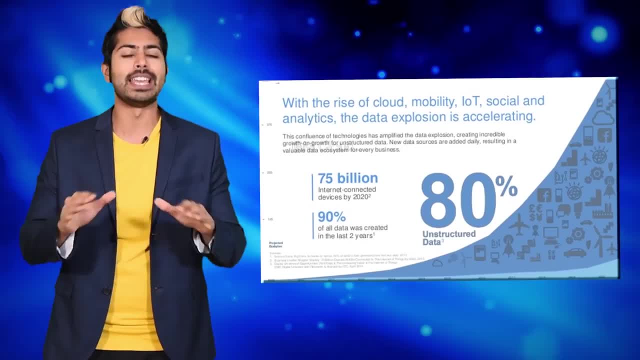 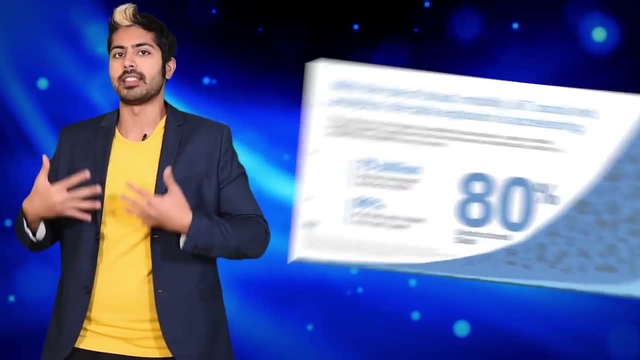 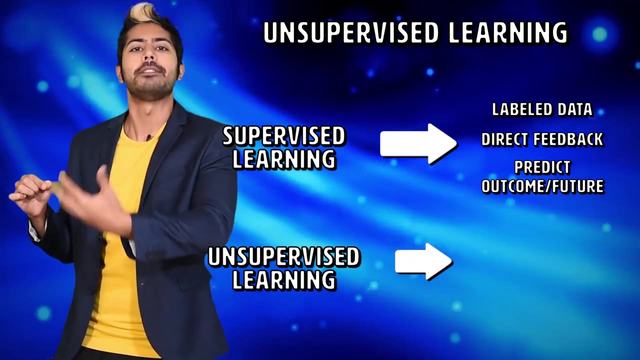 easy to find. In fact, 80% of the world's data is unstructured. The goal of unsupervised learning is to automatically find structure in a data set. This can itself be the goal: discovering hidden patterns in data or a means to an end to learn what the most relevant features. 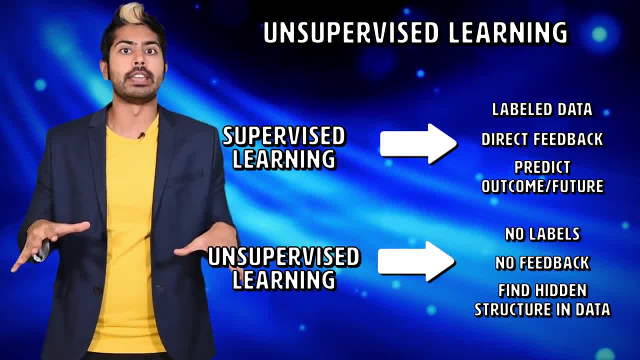 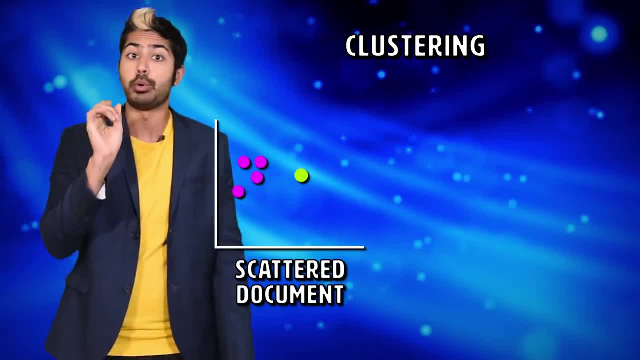 are. We can further subdivide unsupervised learning into different types of techniques. Clustering finds data points similar to each other and groups them together. If we had any kind of population data, whether we were a government organization or a startup with a product like 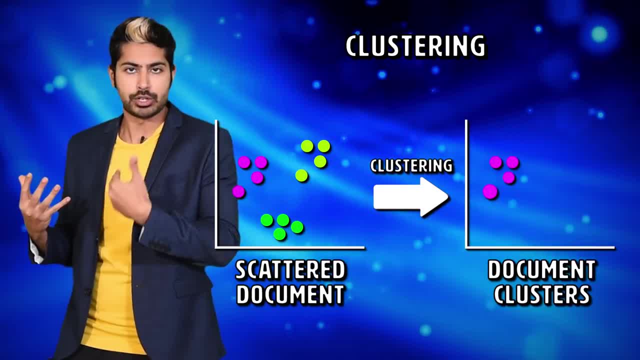 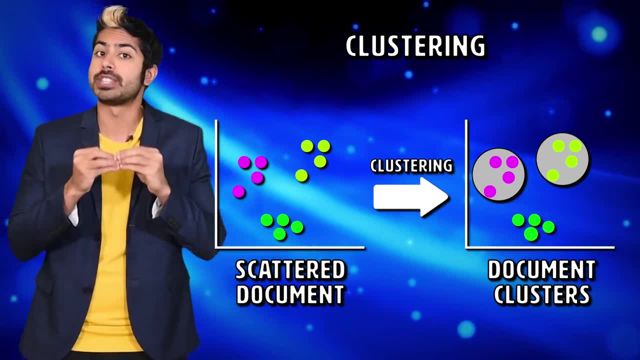 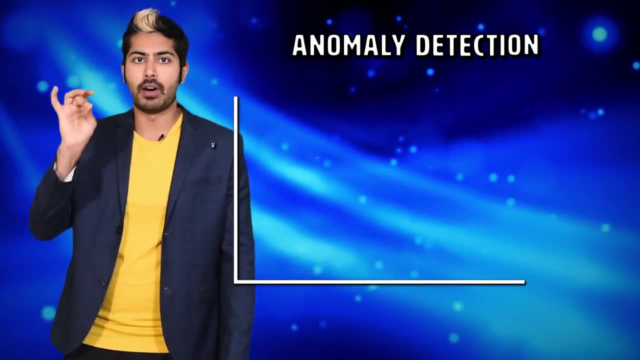 diet water- yes, that's real, Basically anyone trying to reach a certain set of people. we want to segment that population into smaller clusters with similar demographics and purchasing habits so that we could target them most effectively spending our marketing budget. Anomaly detection finds the outliers in a 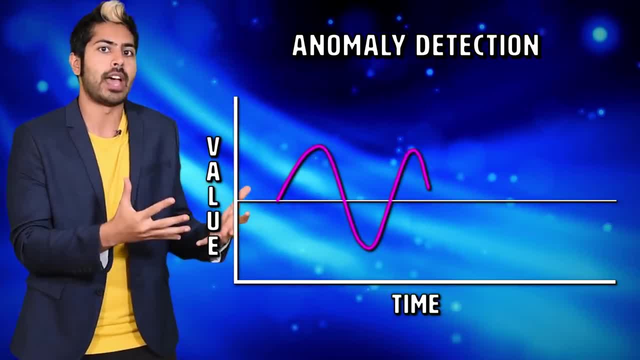 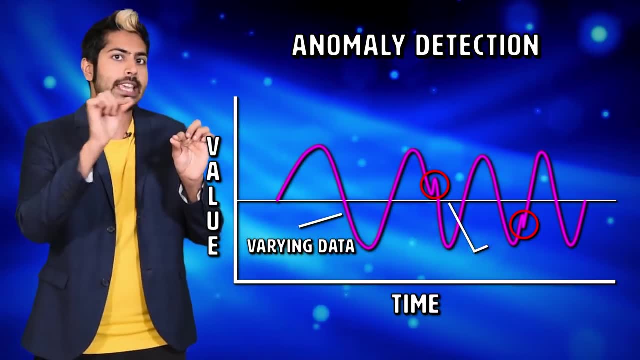 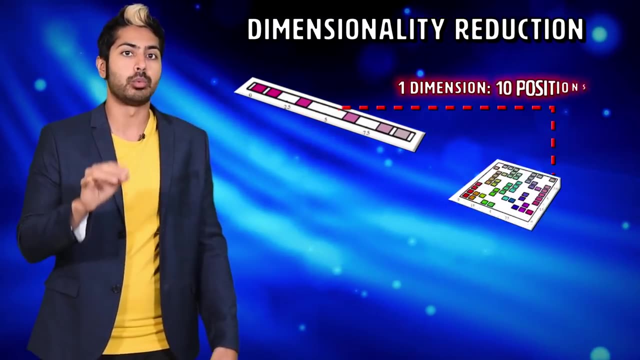 collection of data points. Banks use this to find fraudulent transactions. Association finds correlated features between data points, then lets us infer other features of a given data point. Airbnb uses this to recommend other listings you'd probably like, And dimensionality reduction reduces the number of data points that are used to find fraudulent transactions. 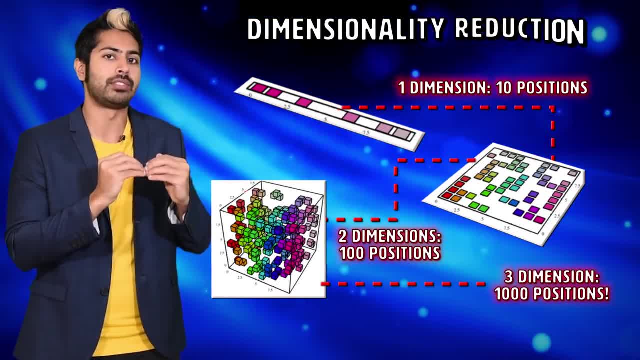 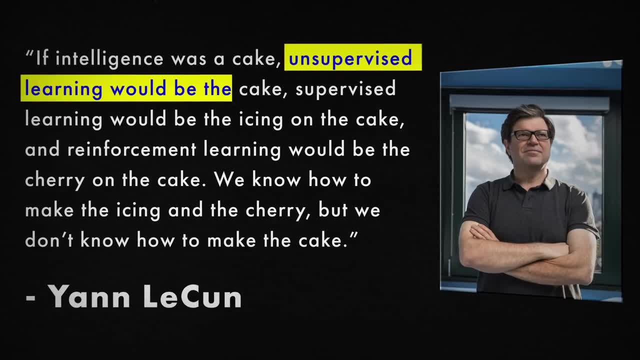 It's also a great way to get a better understanding of what's going on in a data set which makes it easier to visualize and interpret. Yann LeCun, director of AI research at Facebook, puts it best with his quote: If intelligence was a cake, unsupervised learning would be the cake. supervised learning would be. 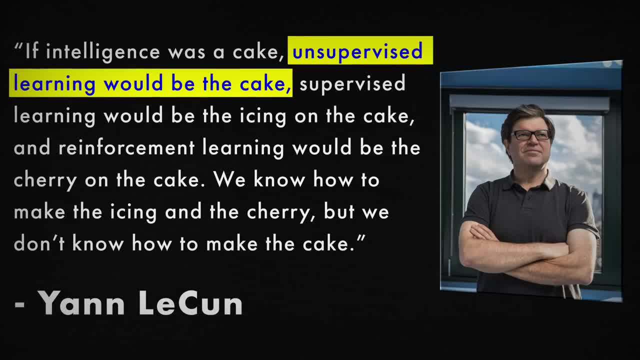 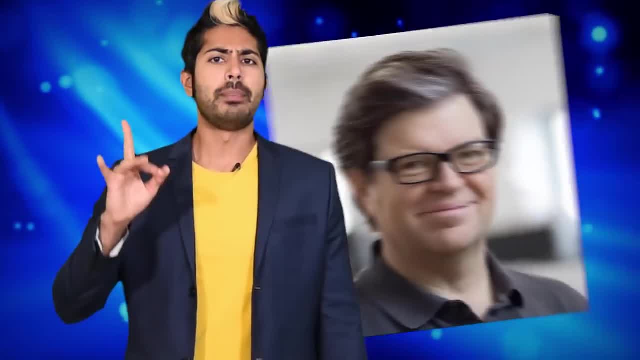 the icing on the cake, and reinforcement learning would be the cherry on the cake. We now know how to make the icing and the cherry, but we don't know how to make the cake. Talk about strange but weirdly effective metaphors. Here's to you, Yann. 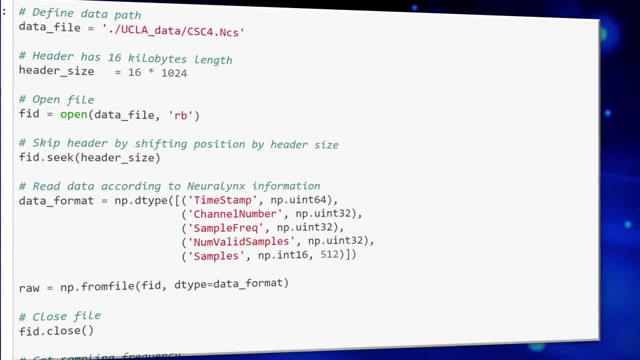 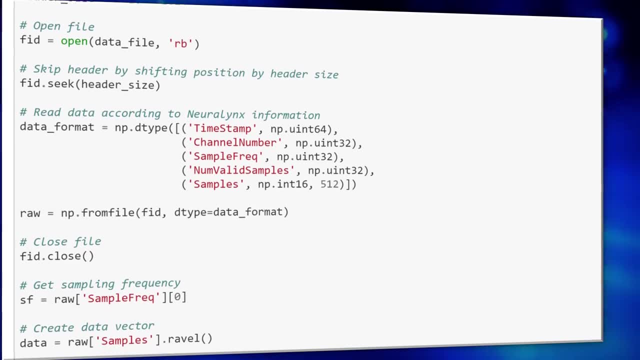 So let's take a look at our data to decide what to do with it. This is a 30 minute long recording of neural data from an epilepsy patient. A set of electrodes were inserted into the brain of this patient to record the activity of neurons in real time. It picked up electrical spikes of neurons. 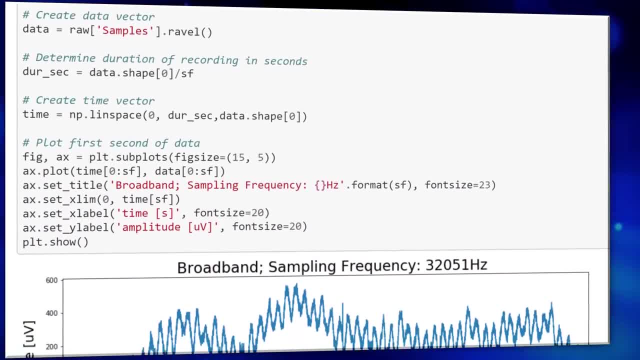 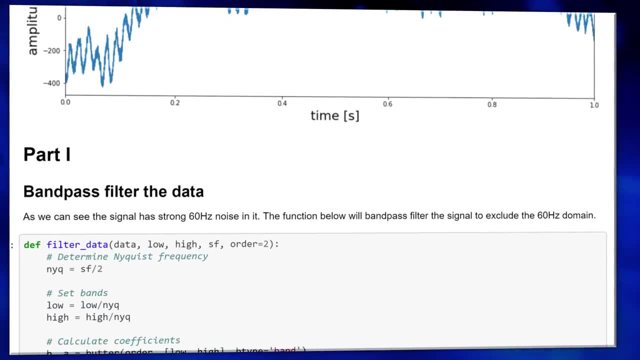 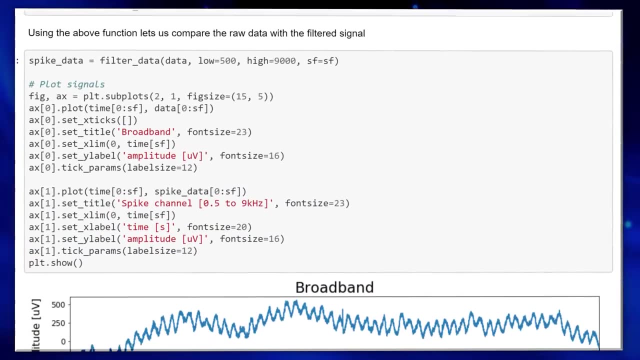 and we can see several features here that relate to the recording device's measurements, like the channel number, frequency and the number of samples. Let's first visualize this data using digital alchemy, aka python. We want to extract spikes from the signal, and to do that we'll find data points in the signal. 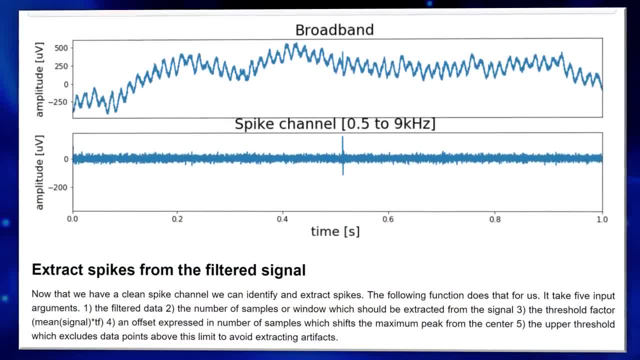 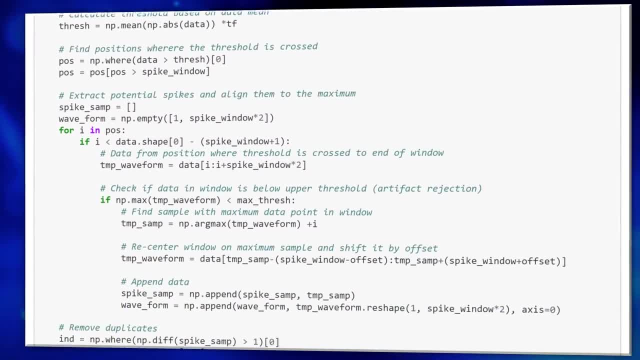 that are above some predefined threshold and align them at their peak amplitude. We can do this with just 100 random spikes and see that there are at least two types of waveforms in the data: One group of spikes with a sharp high amplitude peak and a second group with a 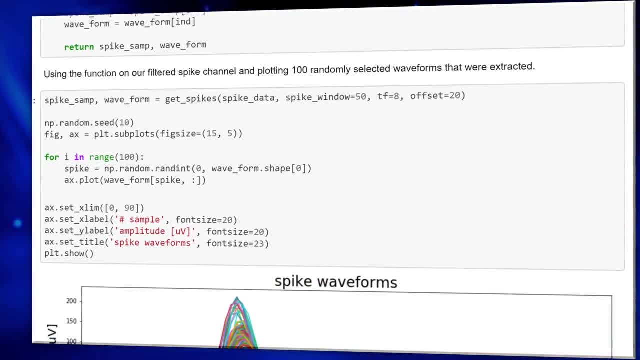 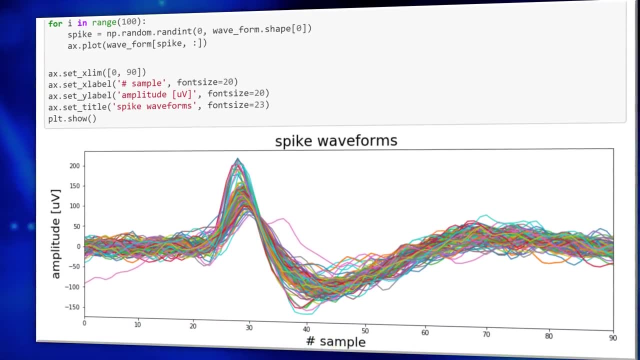 broader initial peak. These spikes were likely generated by more than one neuron. If we can find a way to group these waveforms into different clusters, it will help us figure out which spike corresponds to which neurons, which will help surgeons decide where to perform surgery. 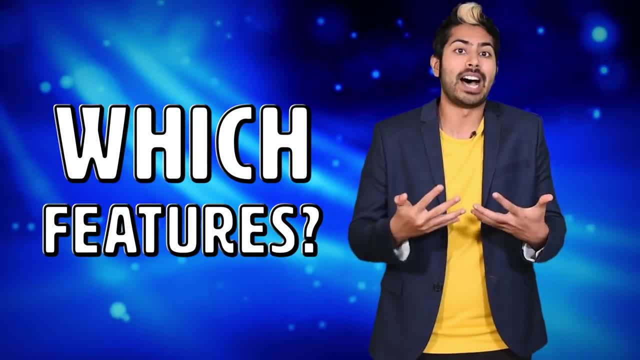 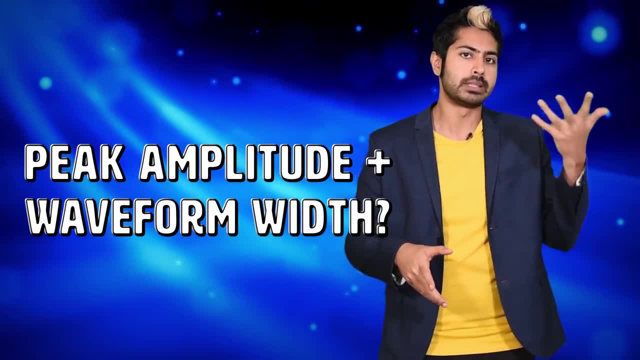 But in order to cluster the waveforms, we're going to need to decide which features to input to our algorithm. One possible feature could be, for example, the peak amplitude of the spike or the width of the waveform, but not all features are equally informative and useful. We need to 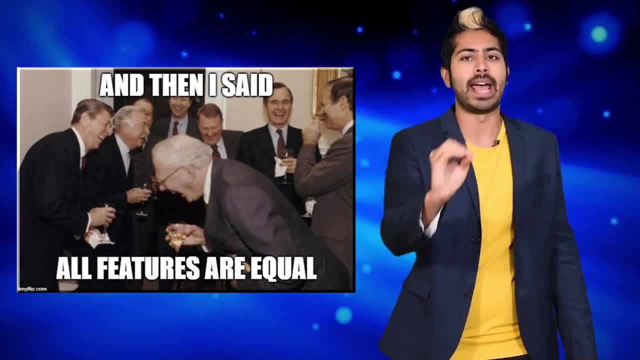 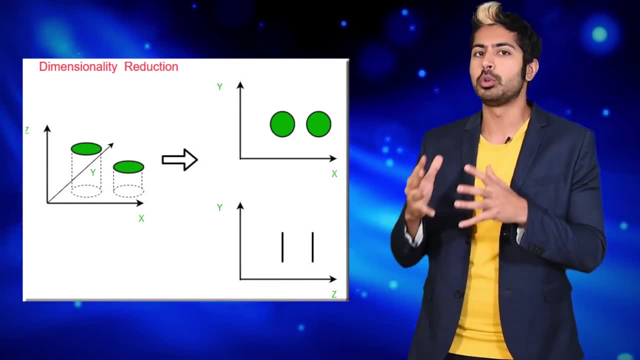 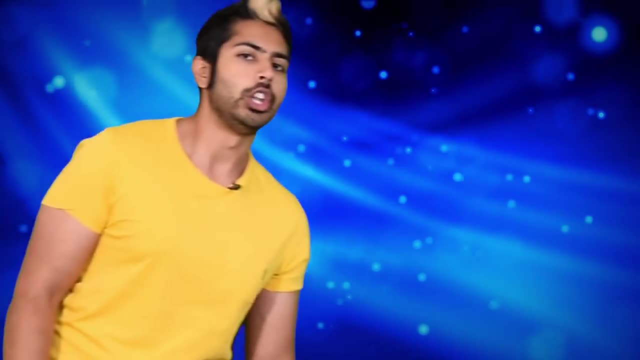 select the features that represent the spike wave shapes the best and get rid of the rest. for our algorithm, We're going to use a type of unsupervised learning called dimensionality reduction, of which there are several techniques, like brute force, No. 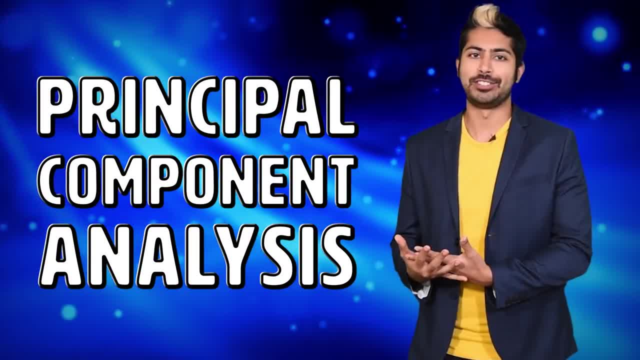 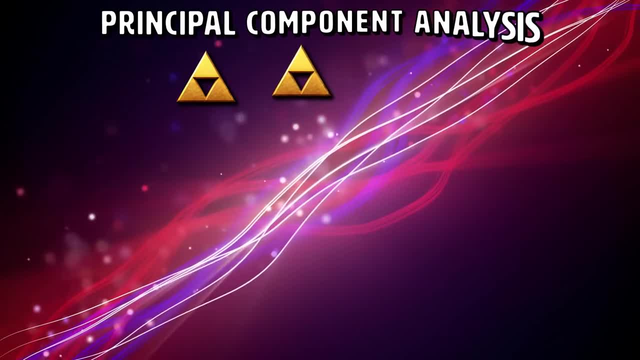 We're going to use a popular one called principal component analysis or PCA. PCA finds the principal components of a dataset. Principal components are the underlying structure in the data. They are the direction where there is the most variance, meaning where the data is most spread. 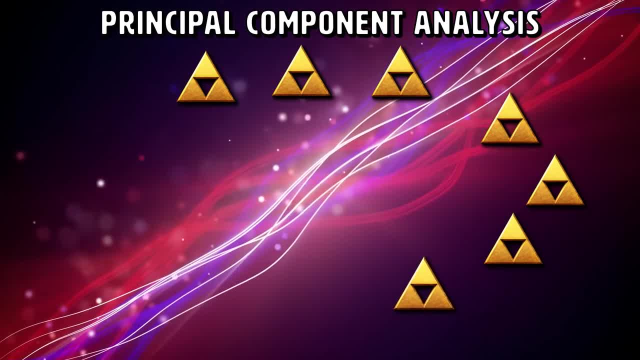 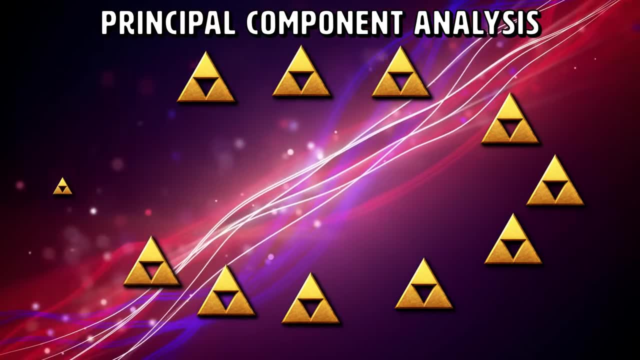 out, It's useful to measure data in terms of principal components rather than on a normal XY axis. Imagine that we had a bunch of data points which we'll denote as triforce symbols, as an ode to the princess, To find the direction with the most variance. 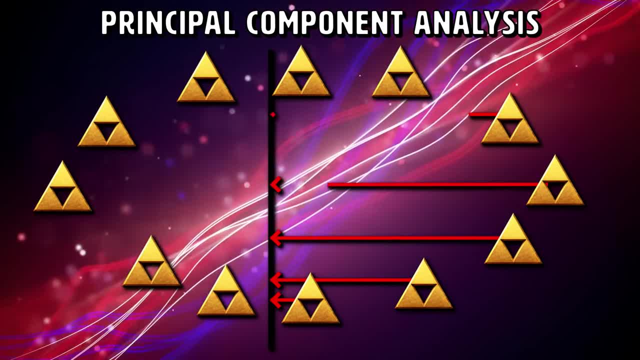 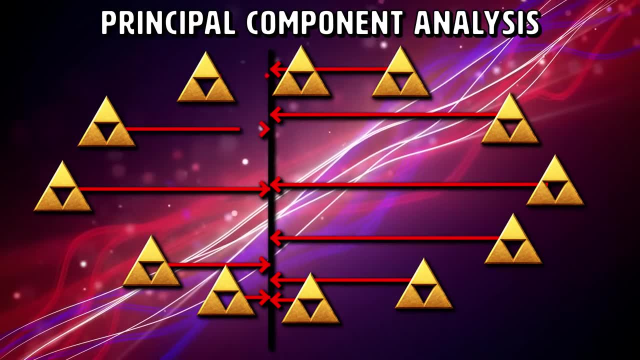 we can find the straight line where the data is most spread out when projected onto it. A vertical straight line with the points projected onto it will look kind of like this: not very spread. so there's a small variance. Likely no principal components. 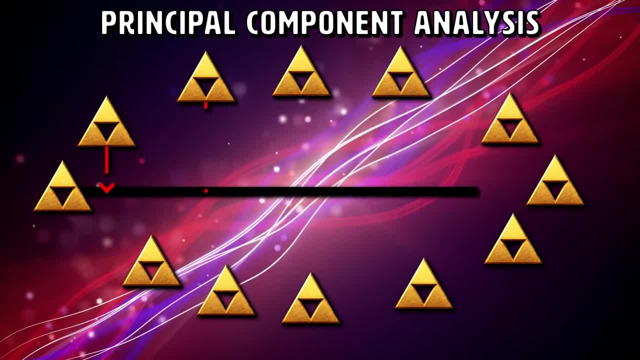 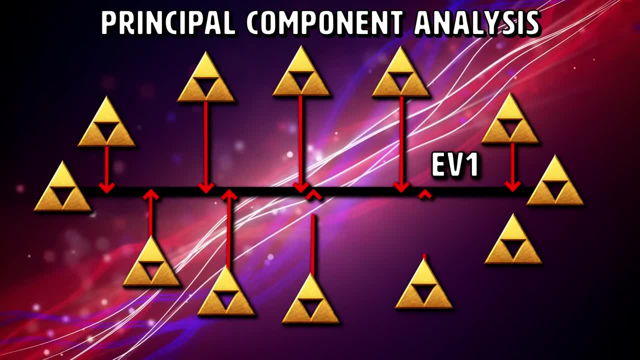 here A horizontal line. however, with lines projected onto it looks way more spread out, a high variance. There's no straight line we can draw that has a larger variance than a horizontal one. Thus the horizontal line is the principal component in this example. 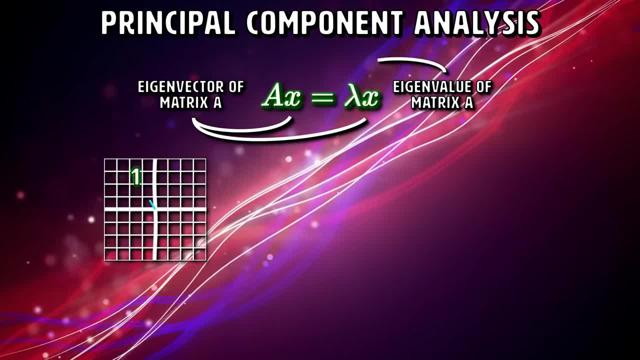 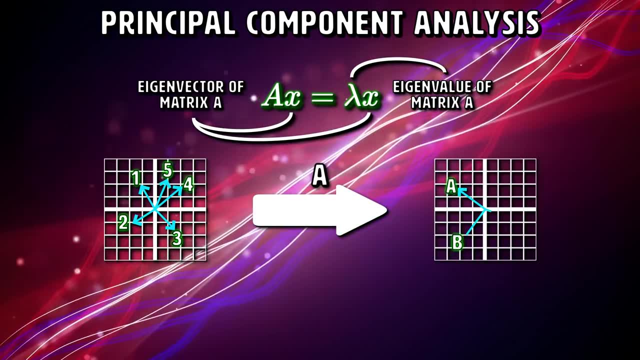 To find principal components. we use linear algebra, one of the mathematical pillars of machine learning. Two concepts here: eigenvectors, which have a direction, and eigenvalues, which are numbers that tell us the direction of the data. We're going to use linear algebra to 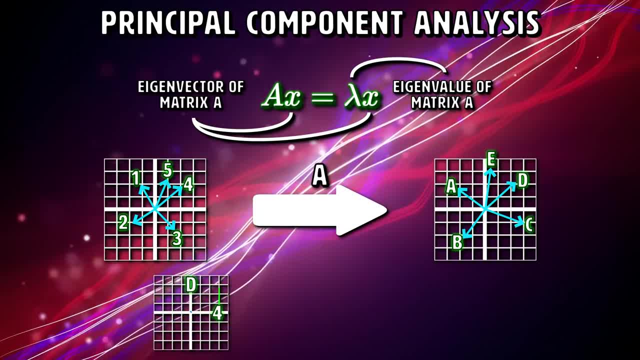 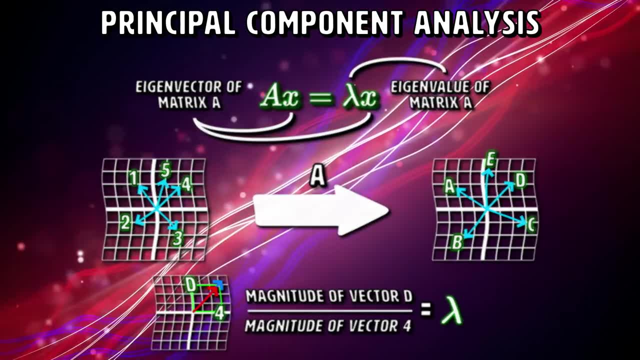 tell us how much variance there is in the data in that direction. These two concepts come in pairs like yin and yang, and the eigenvector with the highest eigenvalue is the principal component In a three-dimensional dataset. there are three variables. Imagine all the data points lie on a. 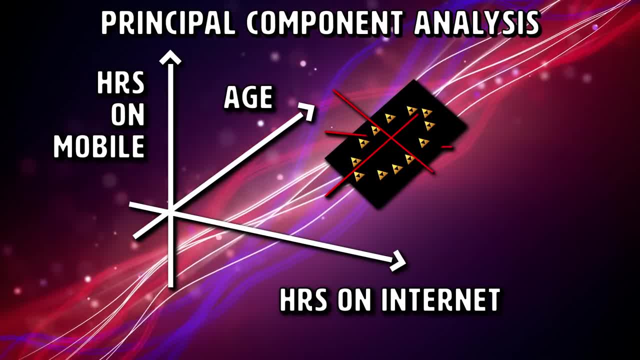 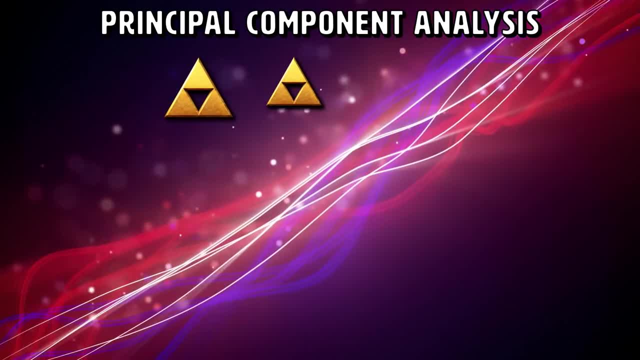 piece of paper-sized plane. in this 3D graph, When we find the three eigenvectors and values, two will have large eigenvalues and one of the eigenvectors will have an eigenvalue of zero If we rearrange our axes. 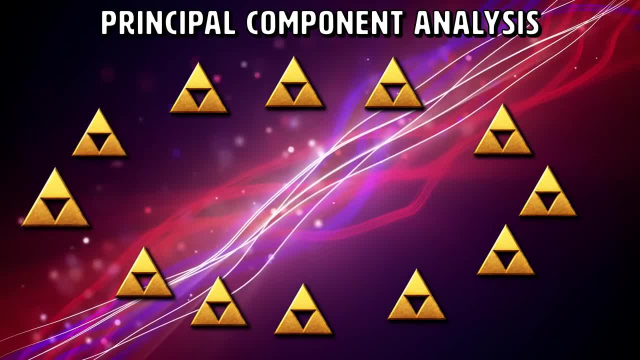 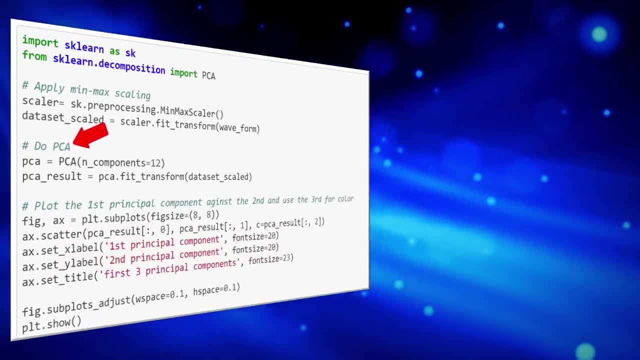 along the eigenvectors rather than the original variables. discarding the third one, we essentially get rid of the useless direction and are able to represent it in two dimensions. We can do this in a single line, thanks to scikit-learn. We just need to specify: 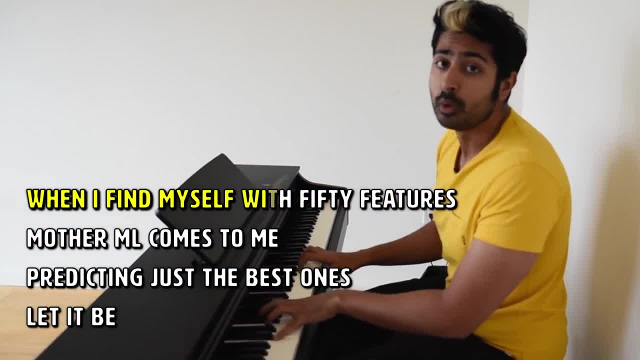 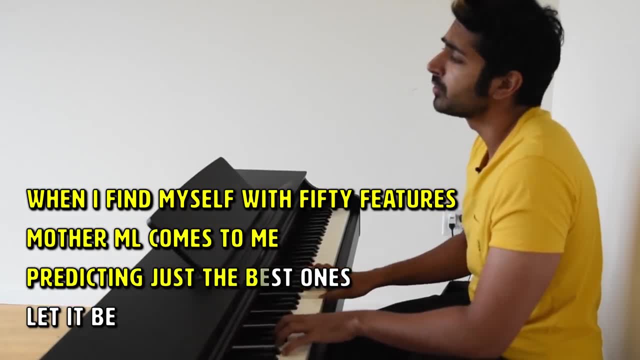 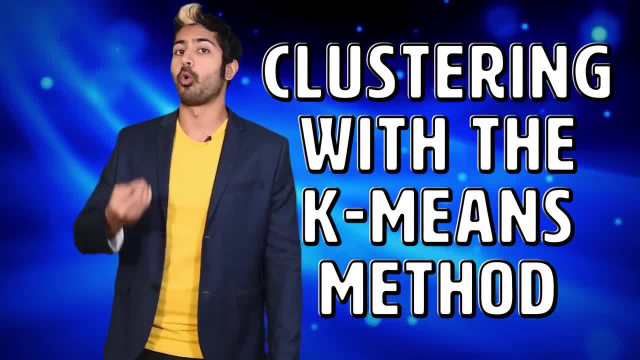 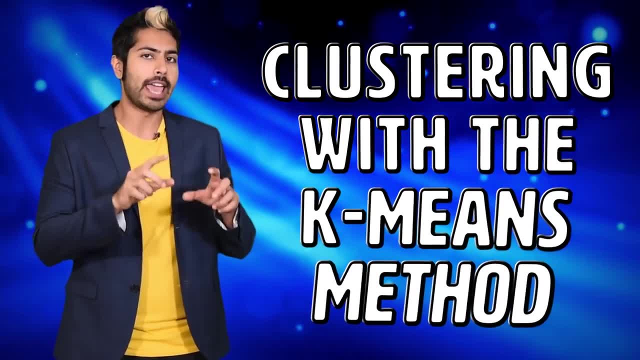 Let it be. Once we've reduced the dimensionality of our data, we're ready to perform clustering, the second type of unsupervised learning. A popular clustering technique is called k-means. First, we choose a number of k random data points from our sample. 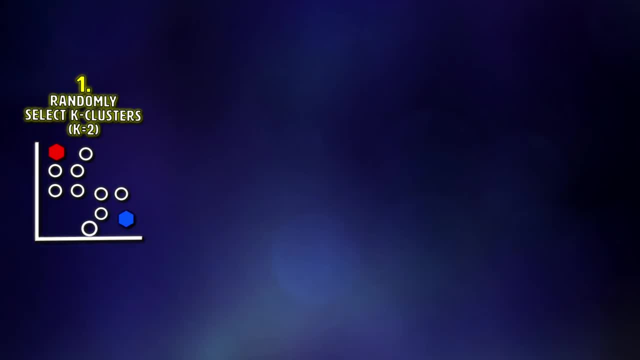 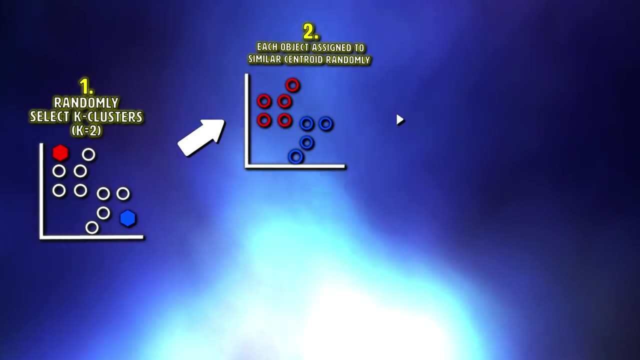 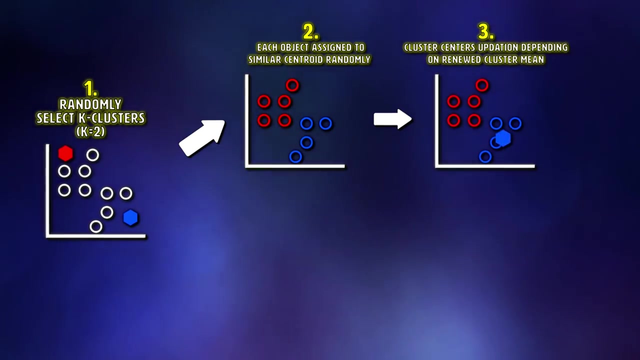 These represent the cluster centers and their number equals the number of clusters. Then we calculate the distance between all the random cluster centers and any other data point. We then assign each data point to the cluster center closest to it. Since we started with random data points, it won't give us a great result. 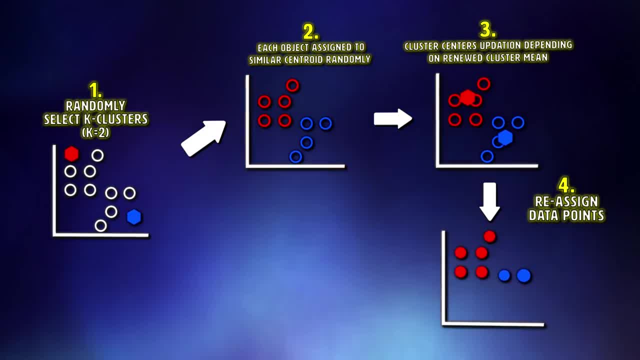 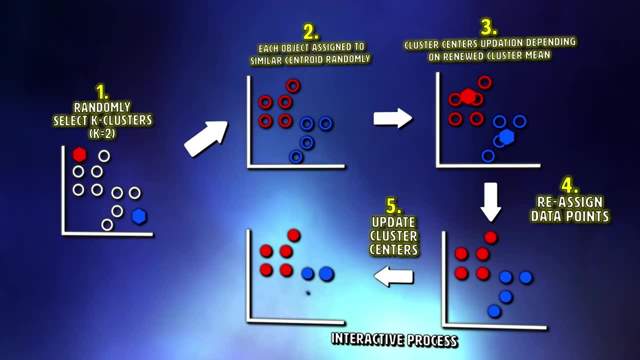 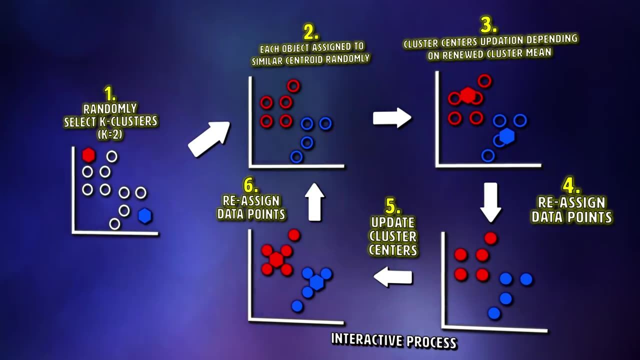 So we repeat the process and instead of using random data points as cluster centers, we calculate the actual cluster centers based on the previous random assignment. This just keeps repeating and with every iteration the data points that switch clusters go down and we arrive at a global optimum. 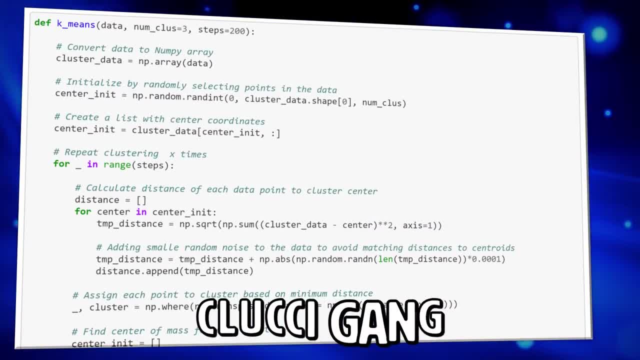 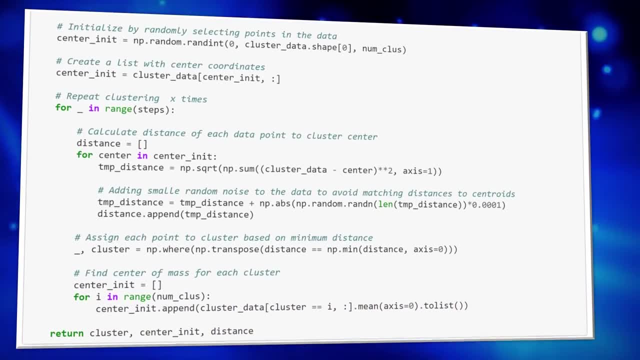 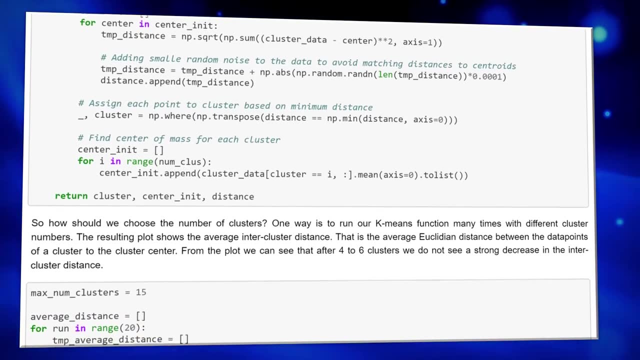 We're now in the cloochie game. A question arises though: how do we choose the number of clusters? We could try running k-means multiple times with different cluster numbers. When we plot the result, we can analyze it to see if we chose too many clusters too. 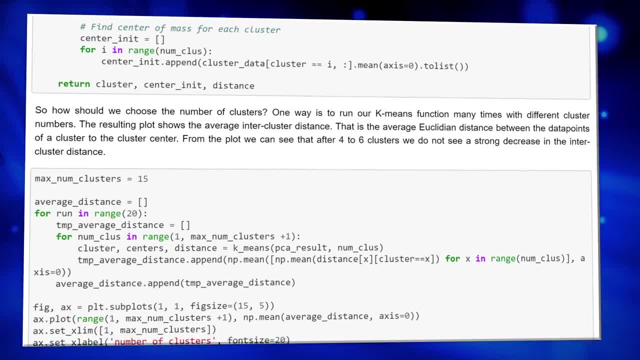 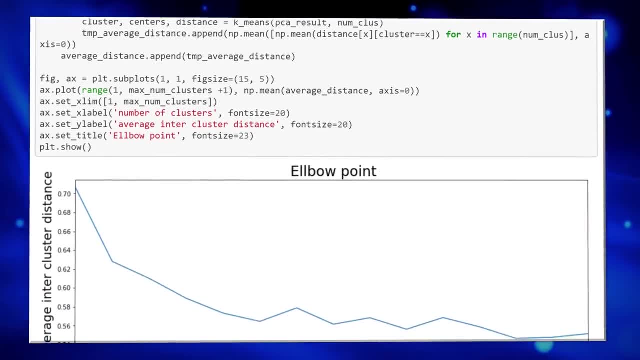 few or just the right amount. based on our domain knowledge, We can expect to find more than two or three separable clusters from a single electrode recording, and our plot seems to confirm this notion. Another way to decide this is to use the k-means method. 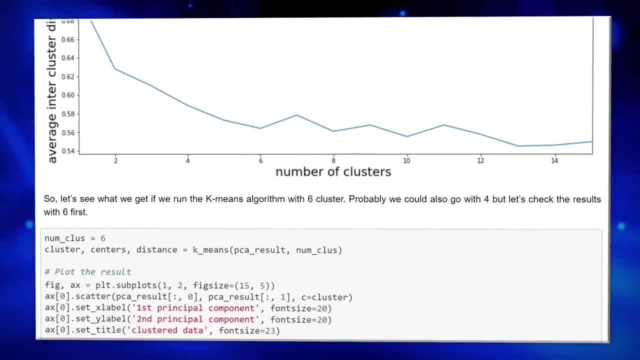 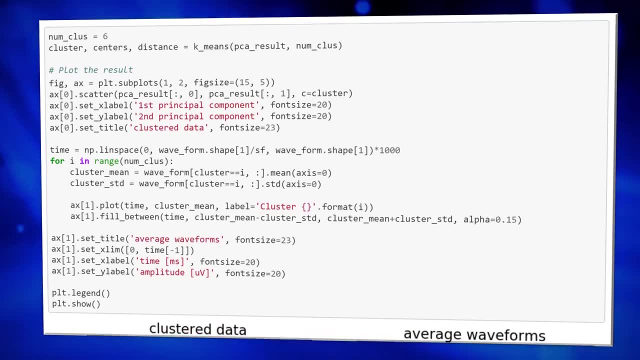 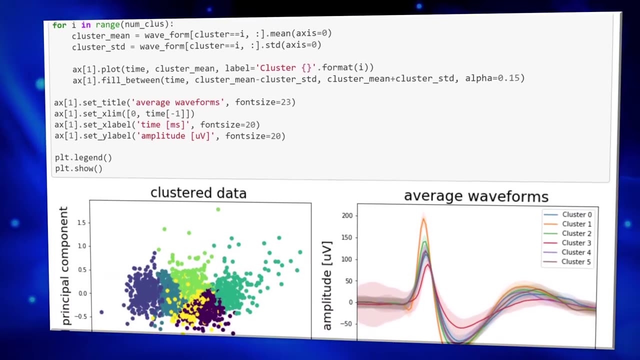 The way this works is to run k-means several times and increase the number of clusters every run, And during every run we calculate the average distance of each data point to its cluster center. The number of clusters increases and the average intercluster distance decreases. 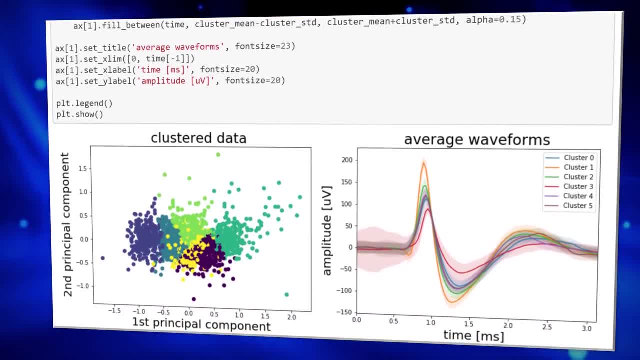 When we reach six clusters, the average distance to the cluster center does not change anymore, and this is called the elbow point. It gives us a recommendation of how many clusters we should run. It also gives us a recommendation of how many clusters we should run.